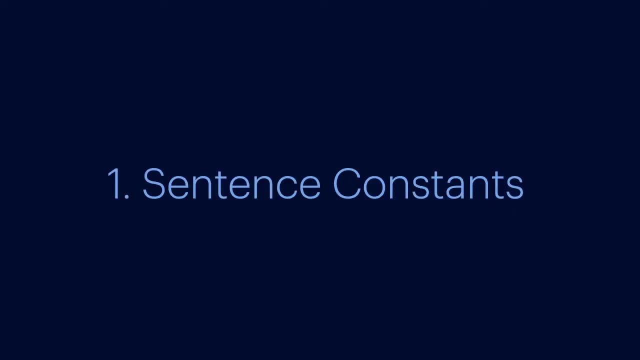 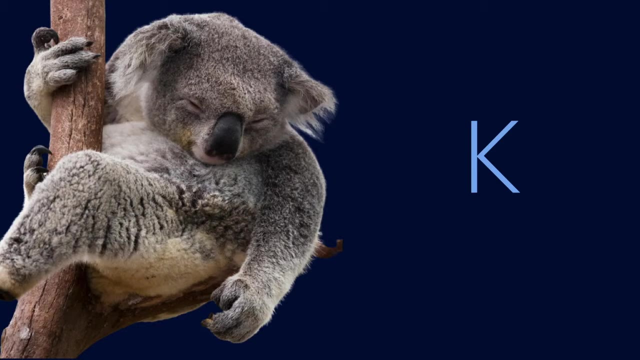 We use a single capital letter to stand for a sentence of English. So the English sentence COWALLAS HAVE FINGERPRINTS becomes K in our formal language. You get to decide what constant stands for what sentence, so you don't have to use the letter K. You could use F instead, or even Z. 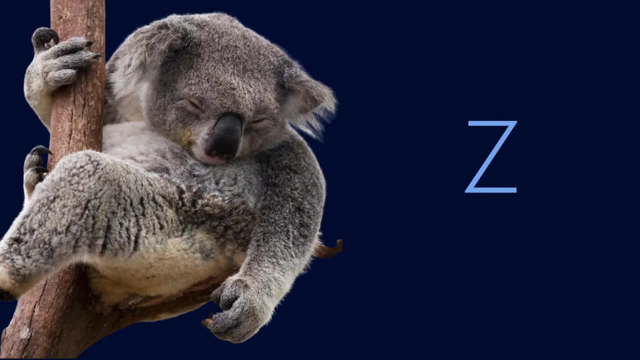 But the point is that in our formal language, the English sentence COWALLAS HAVE FINGERPRINTS is replaced by a constant. A capital letter. 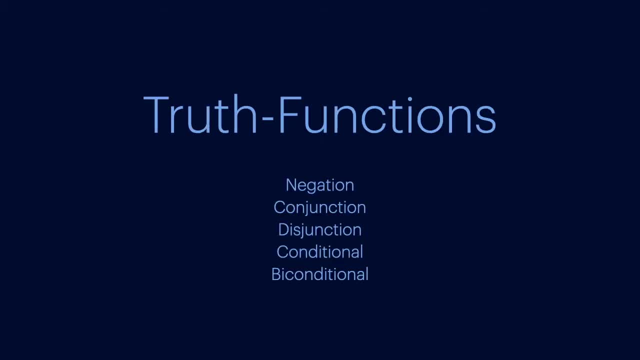 The operators represent the five truth functions. Let's go through each one. This is a tilde. Your textbook may use this symbol instead, or some other notation. That's okay. The point is that it stands for the negation operator. The way to read this operator is 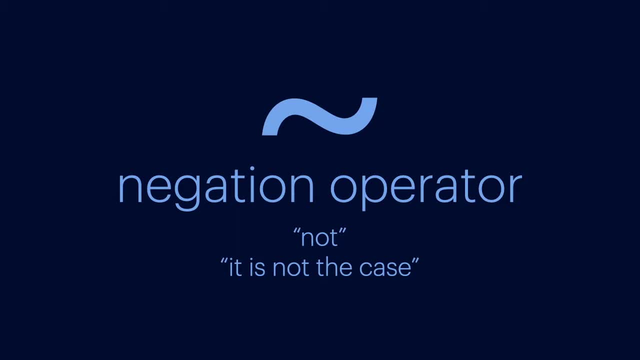 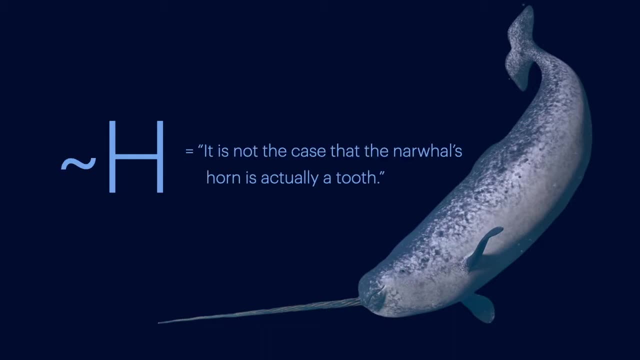 not, or it is not the case. So for instance, this constant standing alone reads, The narwhal's horn is, But now it reads, It is not the case that the narwhal's horn is actually a tooth. 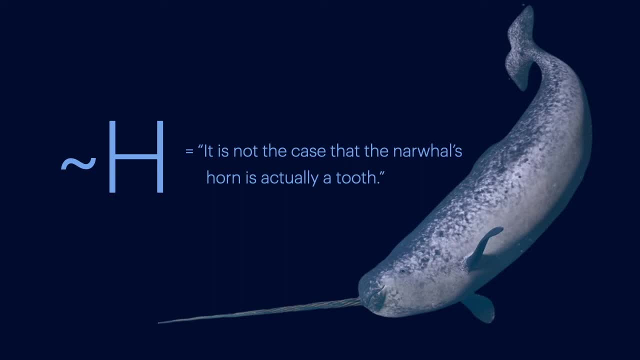 Or more simply, the narwhal's horn is not actually a tooth. 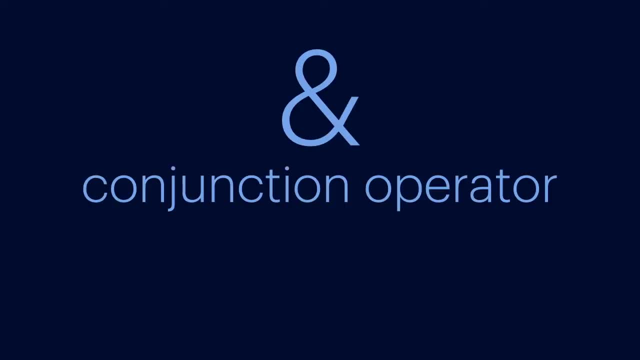 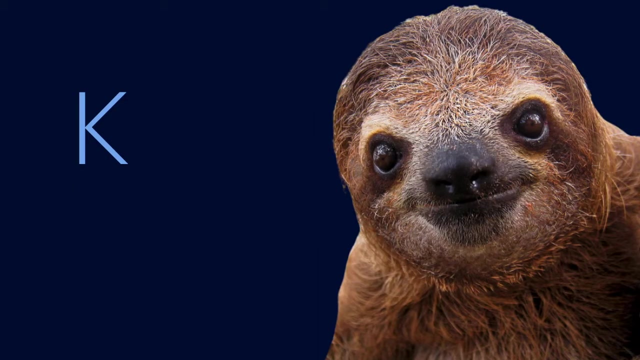 This is an ampersand. It stands for the conjunction operator. Depending on your textbook, this symbol, or even this one, might stand for a conjunction operator. It really doesn't matter. Whatever the exact symbol, it stands for the English AND. Thus, we can take the constant K and the constant S, 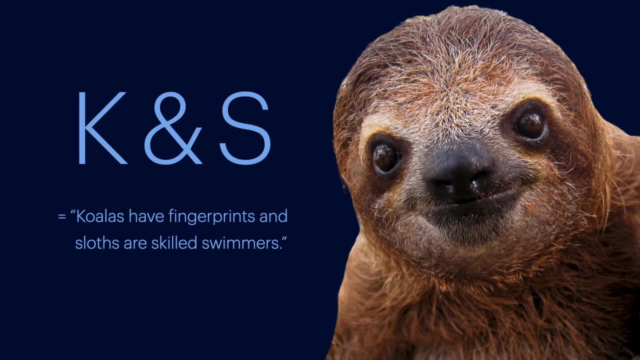 and put them together, with the ampersand, to get, Koalas have fingerprints, and sloths are skilled swimmers. 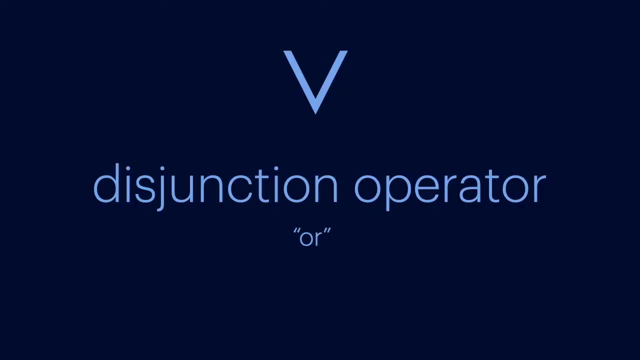 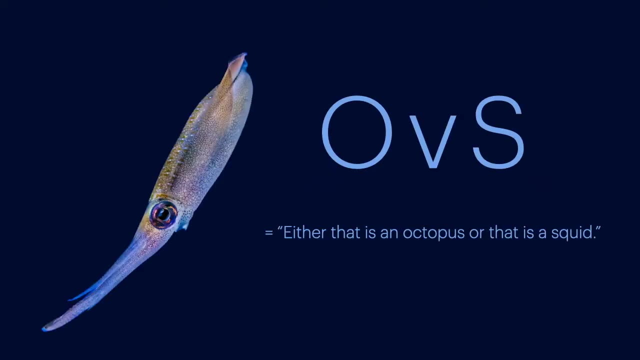 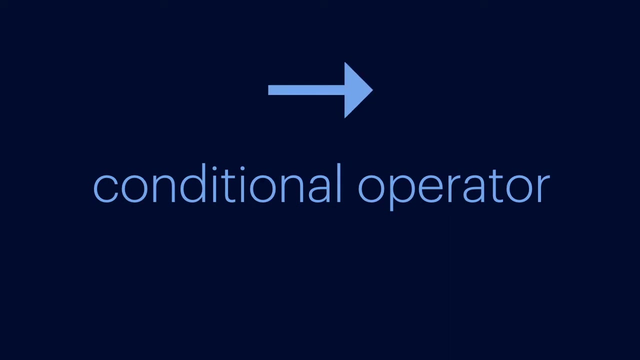 Next, we have the disjunction operator. Its symbol is usually the wedge. This operator reads as the English OR. As in, either that is an octopus, or that is a squid. The horseshoe stands for the conditional operator. Your textbook might simply use an arrow. 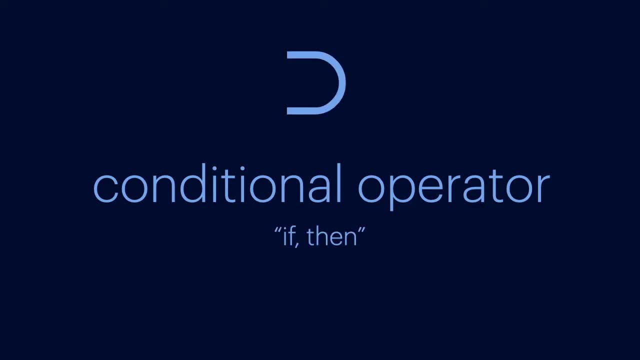 The conditional operator forms if-then sentences. 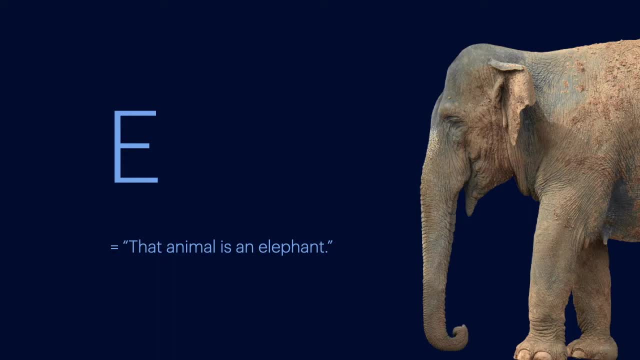 Let's say E stands for, That animal is an elephant. And J stands for, It can jump. So tilde J reads, It cannot jump. Put them together with the horseshoe and we get, If that animal is an elephant, then it cannot jump. 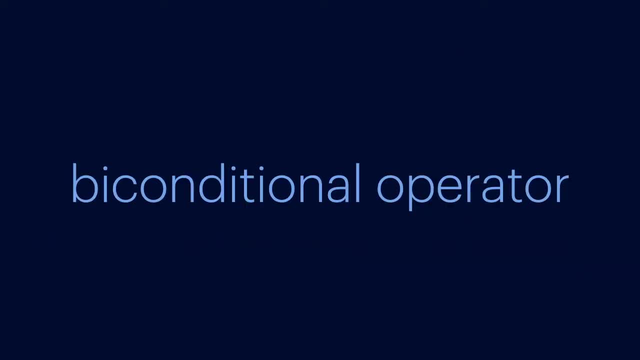 Lastly, we have the biconditional operator. Typically represented by triple bar, or double-headed arrow. 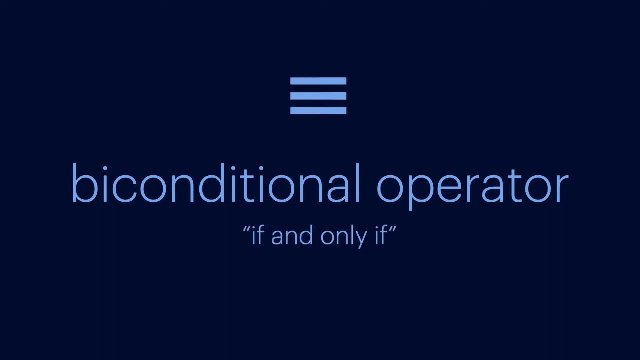 It reads, If and only if. As in, 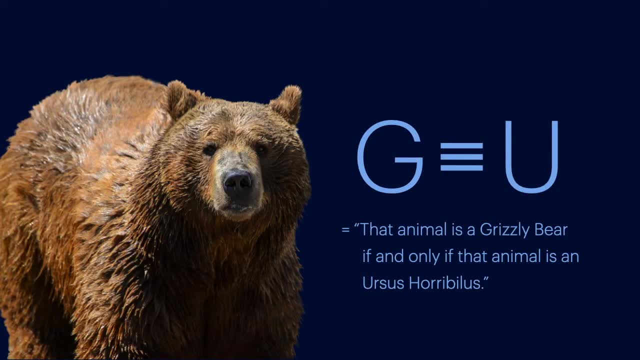 That animal is a grizzly bear. If and only if, that animal is a grizzly bear. If and only if that animal is, a protective animal. 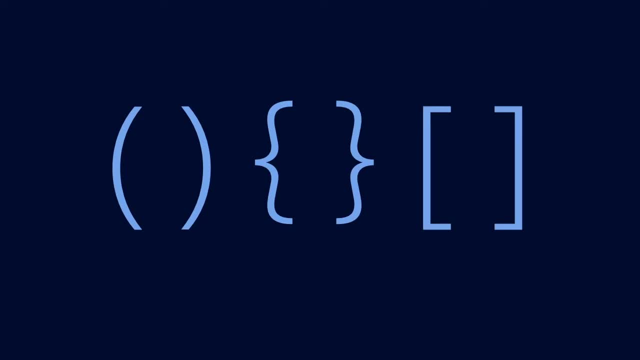 Lastly. Our formal language has parentheses, braces, and brackets. 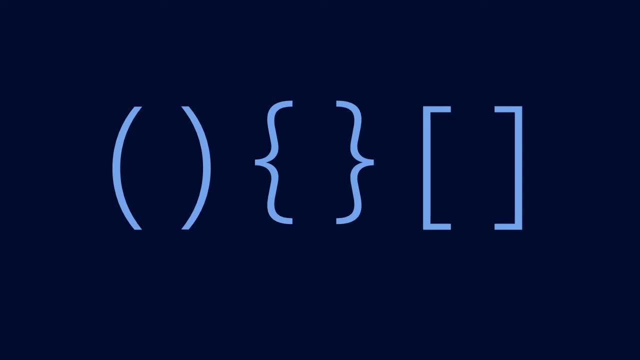 Students sometimes worry about the differences between them, but it doesn't really matter. These are all just options for grouping, when you need to do so. 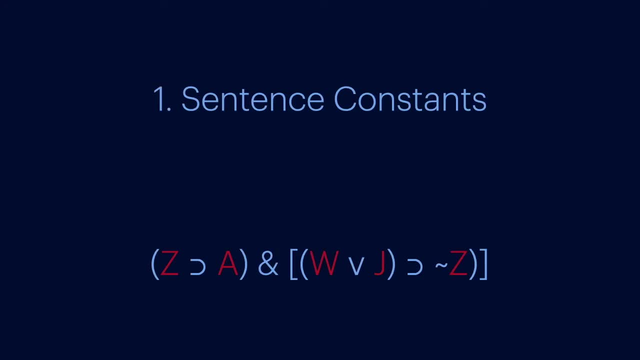 More on grouping later. So that's it. 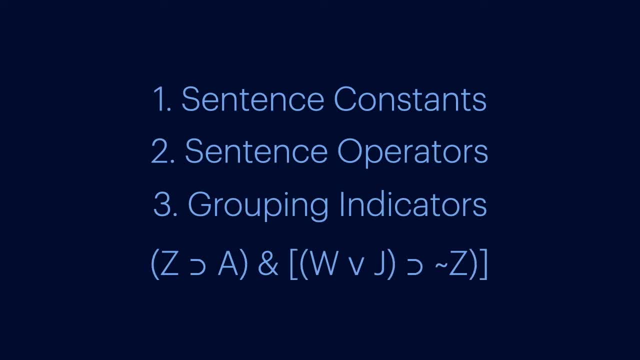 Our formal language is made up of constants, operators, and grouping indicators. Pretty simple, right? Now we just need to know how to put them all together properly. 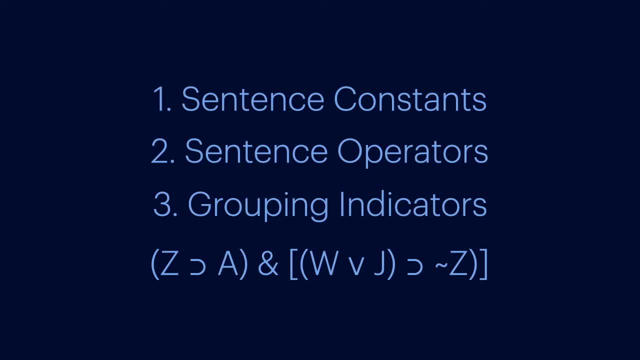 Let's call a correctly constructed sentence of our formal language a well-formed formula, or WIF for short. There are only three rules of grammar for our language, and they're pretty easy. 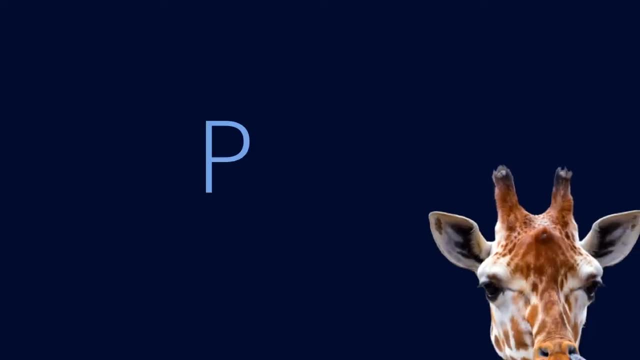 This is a WIF. It says, Giraffes' tongues are purple. 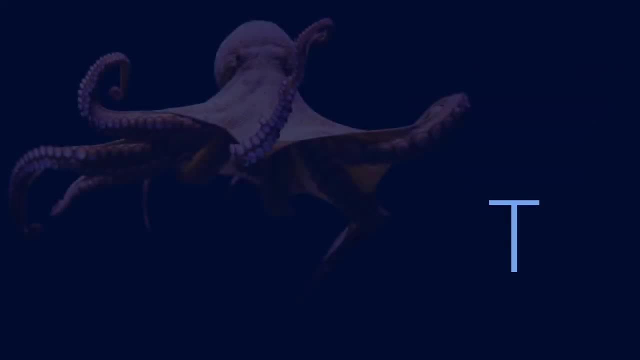 And this is a WIF. It says, Octopuses have three hearts. 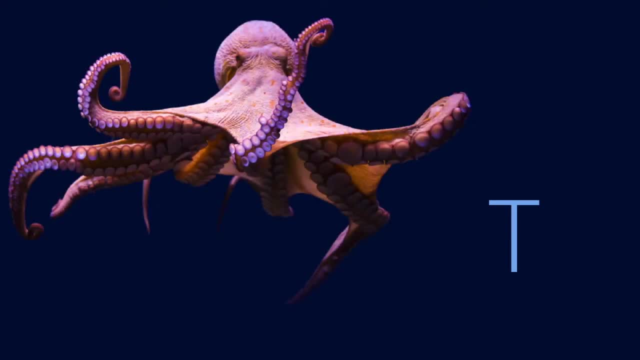 So the first rule of our language is simple. If you have a constant by itself, it's a WIF. 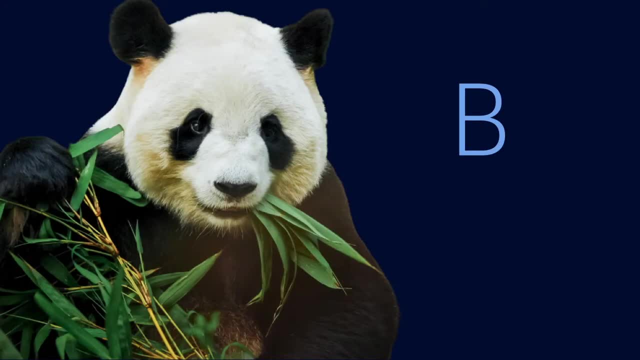 This is a WIF. It says, Pandas only eat bamboo. So this is a WIF too. 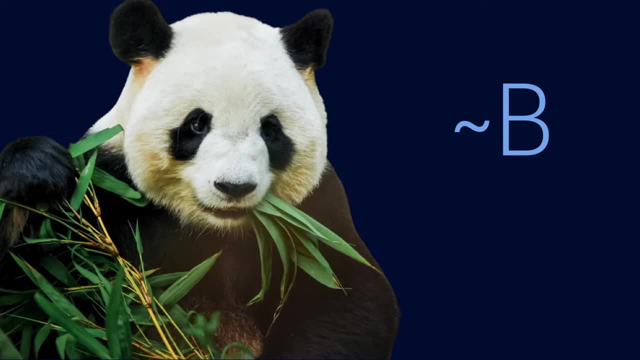 It says it is not the case that pandas only eat bamboo. Or if you prefer, pandas do not only eat bamboo. 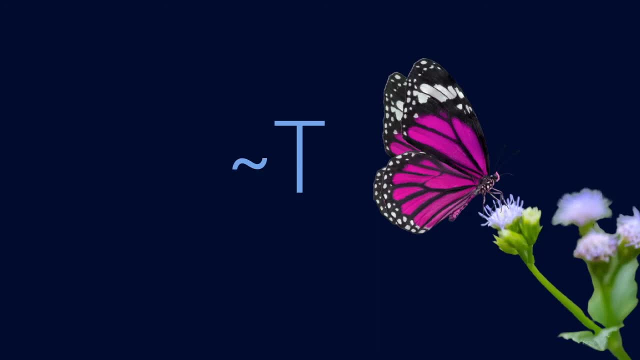 This is a WIF because it's a sentence letter standing alone. This is a WIF. It says, Because it's a sentence letter tagged with a negation operator. 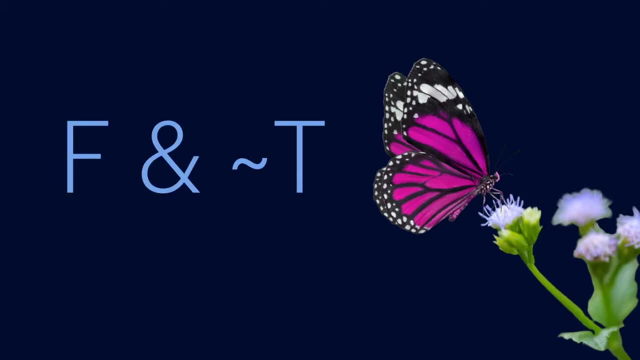 So this is a WIF. It reads, Here's another. If it's a honey badger, then it's a tough creature and immune to venom. 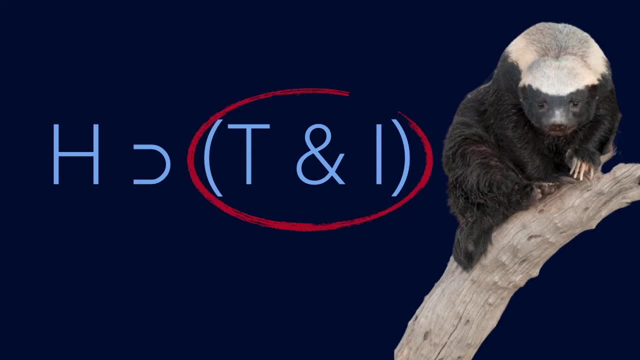 This is a WIF. This is a WIF. So this grouping is a WIF. And this WIF is connected to this WIF with the conditional function. So it's a WIF. And just like that, we're done. Our formal logical language is pretty simple. 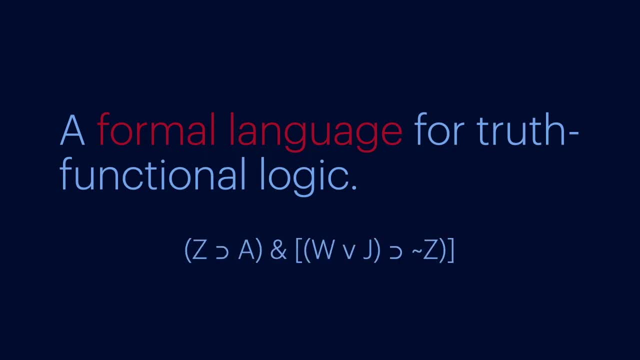 It's made up of constants, operators, and grouping indicators. And we put them together according to three simple rules of grammar. Let's close with a few examples to test your understanding. Ready? Is this a WIF? No. 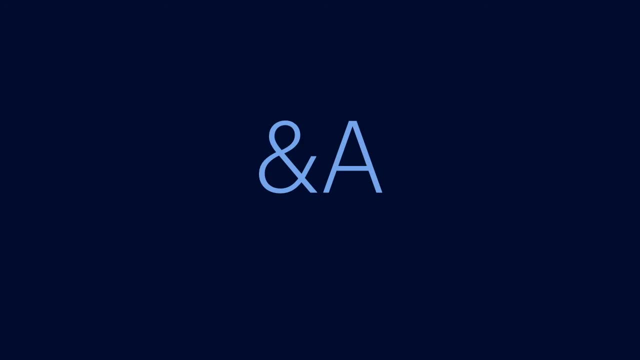 The conjunction operator can join two WIFs to create a new WIF. But it can't just be tagged on the front of a WIF. So this is not a WIF. How about this one? Is it a WIF? No. 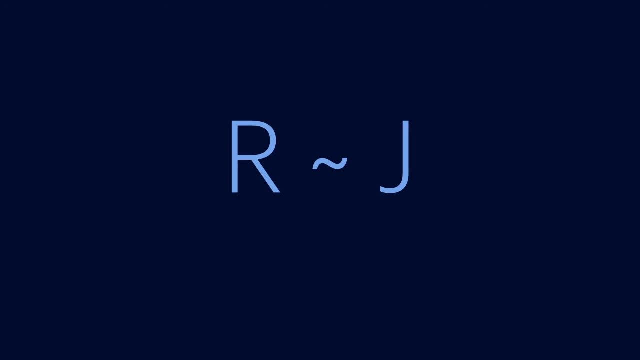 You can tag a WIF with a negation function and the result will be a WIF. For instance, this is a WIF. 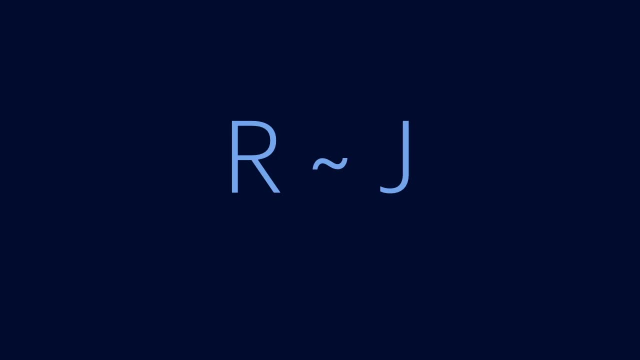 But you cannot join two different WIFs with the negation function to create a new WIF. Here's another. WIF or not a WIF? It's a WIF. 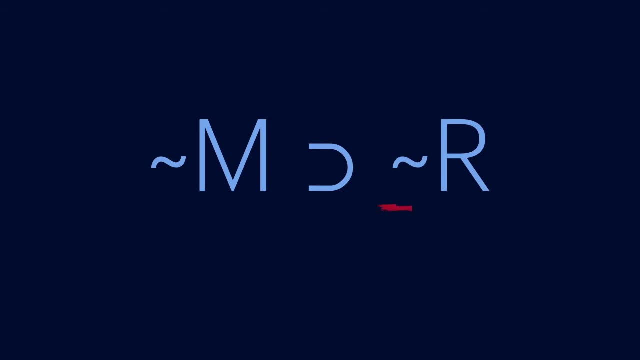 Because this is a WIF. And so tagging it with the negation operator is a WIF. Same goes here. So these are WIFs. 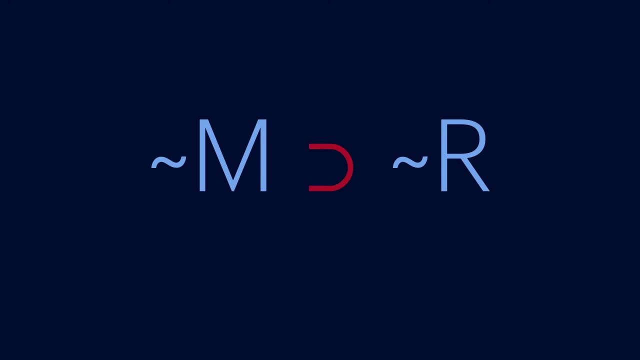 And when you join a WIF to another WIF, using the conditional operator, the result is a WIF. 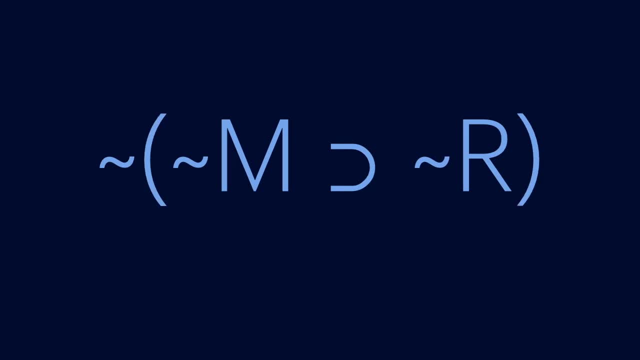 Now here's a tough one. Is this a WIF? Yes. 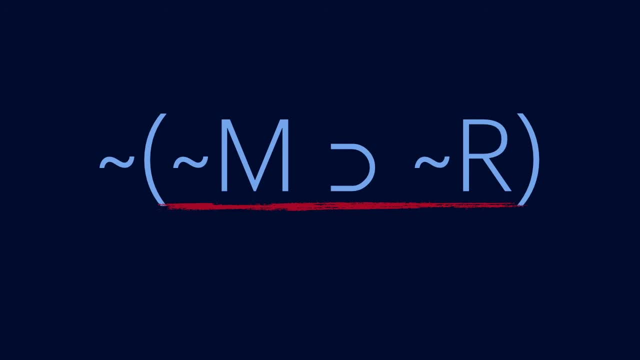 We just said this is a WIF. And according to our rules, you can tag a WIF with the negation function, and the result will always be a WIF. 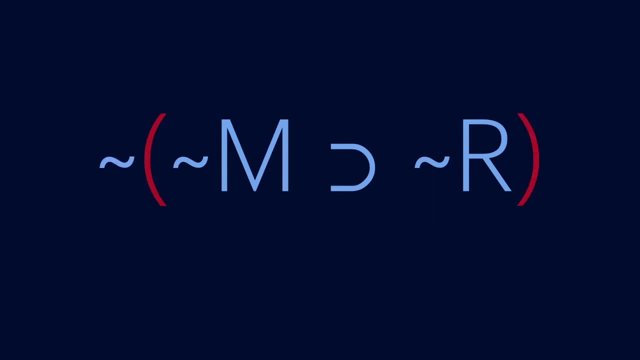 The parentheses show that the negation operator is tagged onto this WIF. 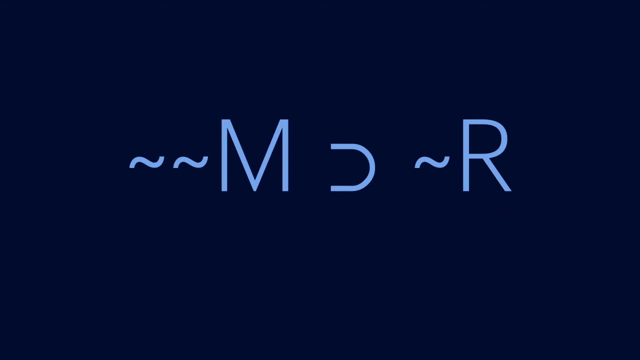 But what if we didn't use parentheses, and just tagged on another negation operator like this? Is it a WIF? Yes. 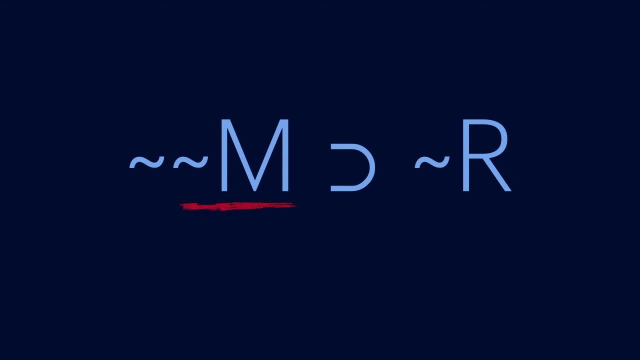 This is a WIF because it's a constant standing alone. This is a WIF because a WIF tagged with a negation operator is a WIF. And since we just said this is a WIF, this is a WIF too. 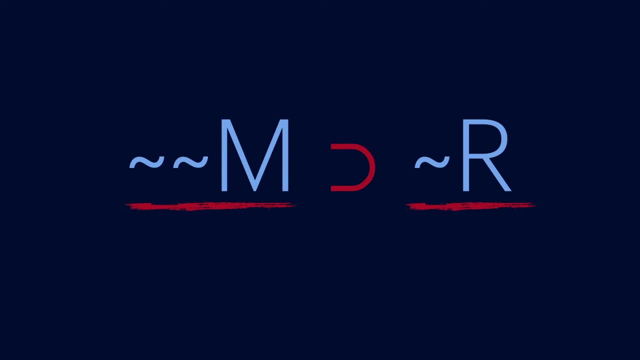 Of course, this is a WIF over here, and the two of them are joined with the conditional operator. So the end result is a WIF. 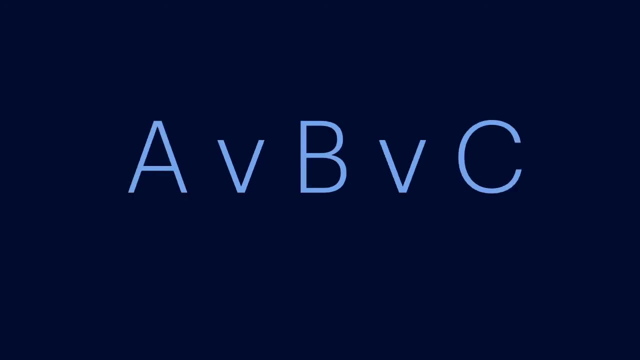 Last one. Is this a WIF? No. 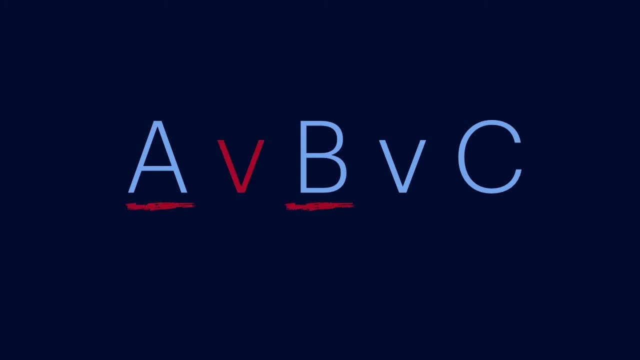 Our rules of grammar say that you can connect a WIF to a WIF using disjunction. But the rules don't allow us to connect a WIF to a WIF to a WIF.